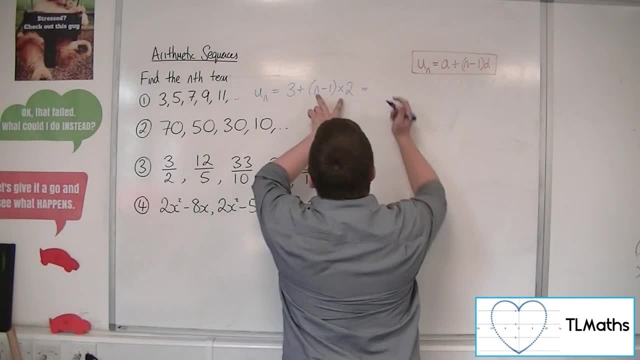 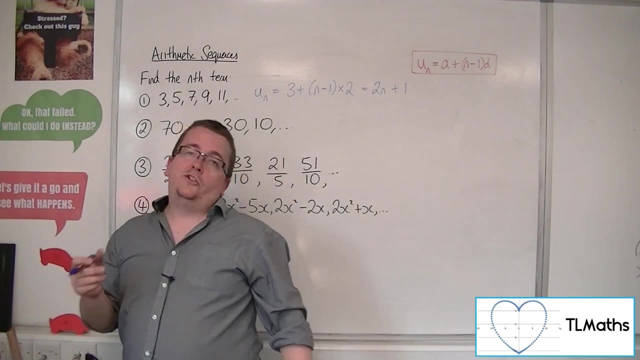 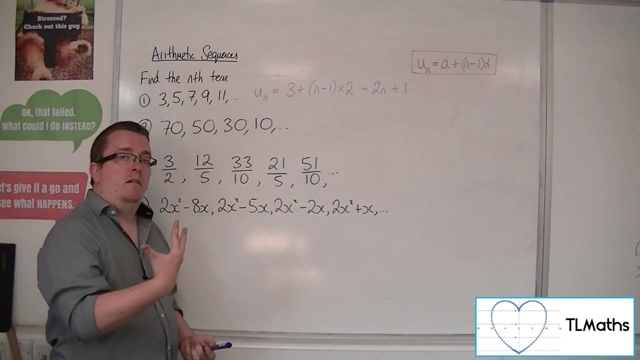 Now I could expand that out, because I'm going to get two, lots of n. I've got a 3, take away a 2, which gets me the 2n plus 1.. So it's precisely the same as what I spotted initially, but it gives you a more formal way of building the nth term up. 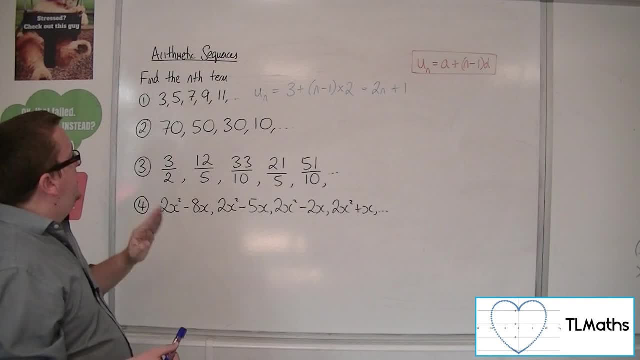 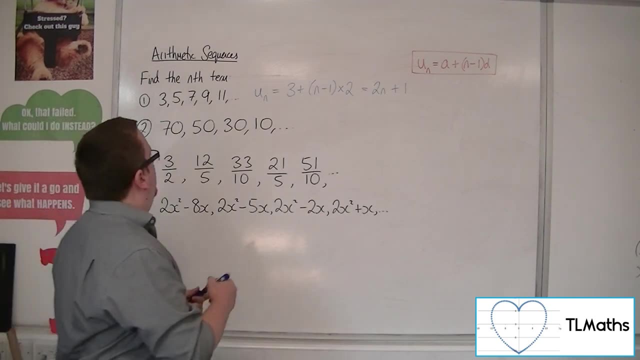 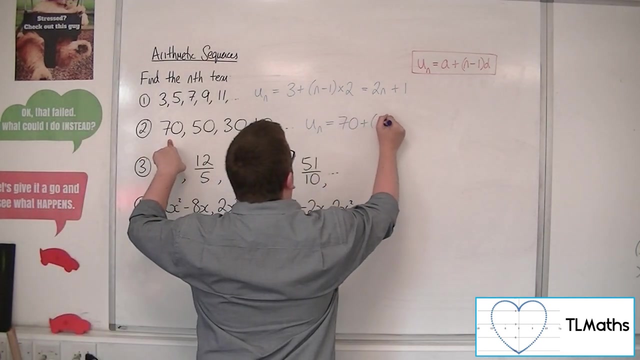 So let's have a look at number 2. We've got 70,, 50,, 30,, 10. We'd be thinking, We'd be thinking, that this would be minus 20n plus 90. Okay, So un is equal to first term, which is 70, plus n minus 1, times by the common difference minus 20.. 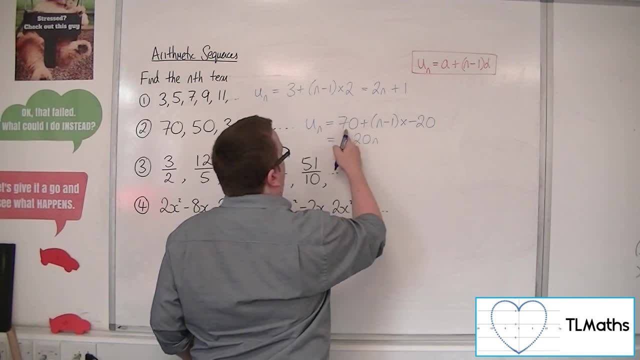 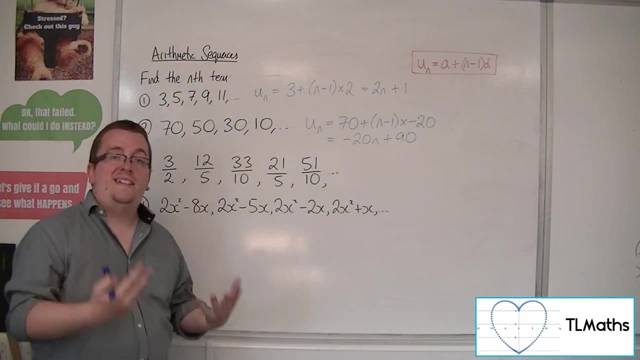 So we've got minus 20n, Then we've got 70 plus 20,, so plus the 90. And that is exactly what we had anticipated it to be. Now, with number 3, I haven't made it so obvious- 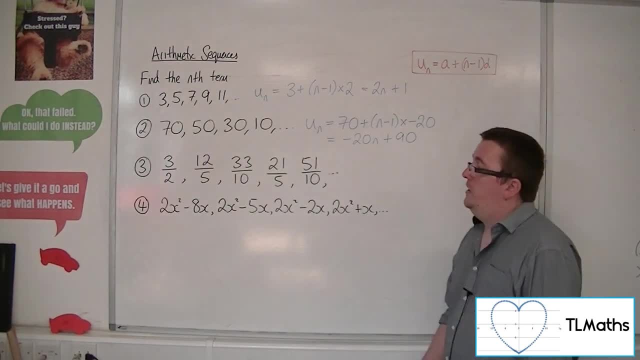 Okay, Now we've got 3 halves, 12 fifths, 33 tenths, 21 fifths, 51 tenths. You'd be hard pushed to actually think that this was an arithmetic sequence. Okay, But if we do 12 fifths, take away 3 halves, we get 9 tenths. 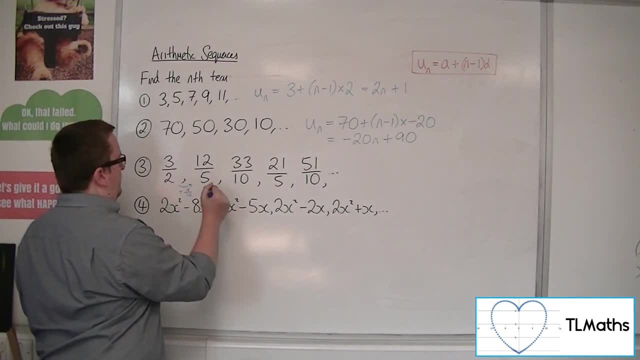 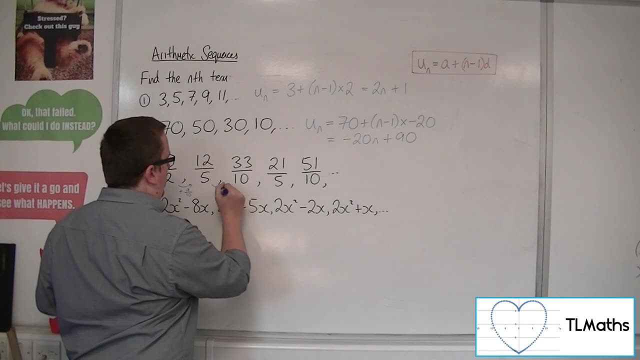 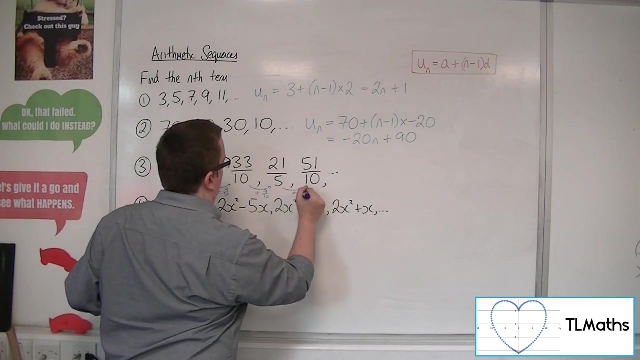 So we are adding on 9 tenths here. Okay, 33 over 10,. take away 12 over 5, is also 9 tenths. So each time we're actually adding on 9 tenths Okay. 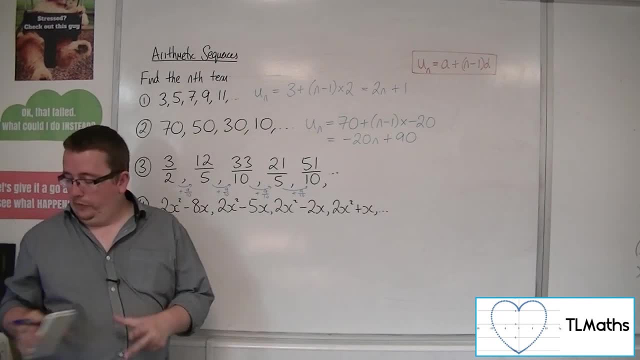 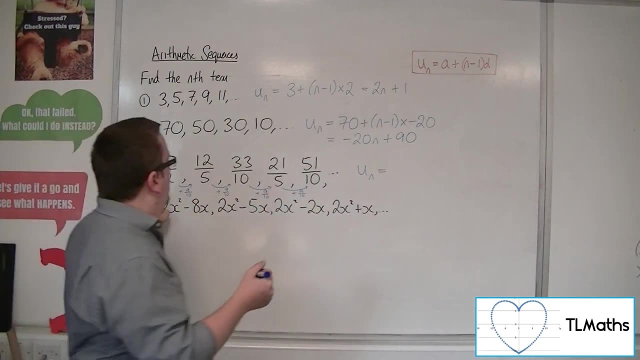 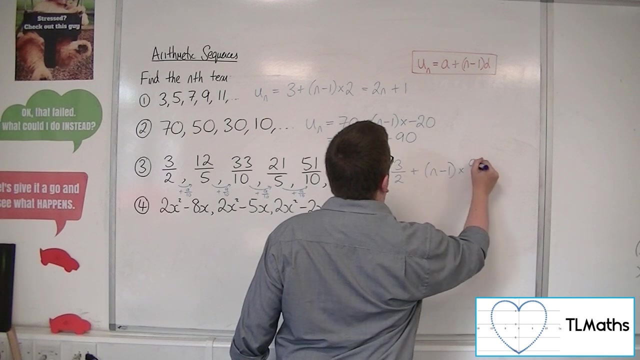 And you can check that for the rest. But that gives us the common difference. So the nth term is the first term: 3 halves plus n minus 1.. Times by the common difference: 9 tenths. So multiplying this through we've got 9 tenths n. 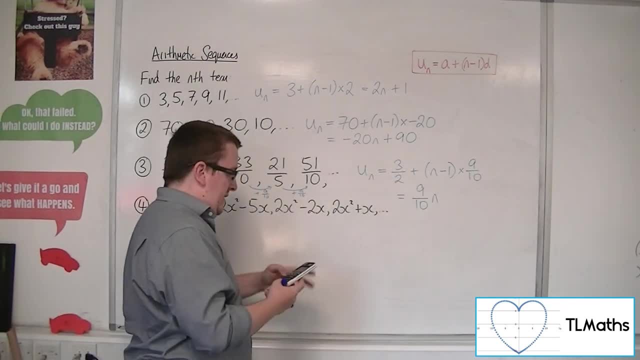 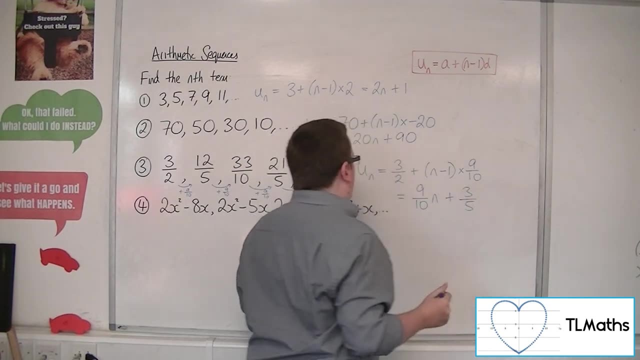 We've then got this: 3 halves take away 9 tenths. So 3 halves take away 9 tenths is 3 fifths. So if we try this out with the fifth term, we're going to have 45 over 10..